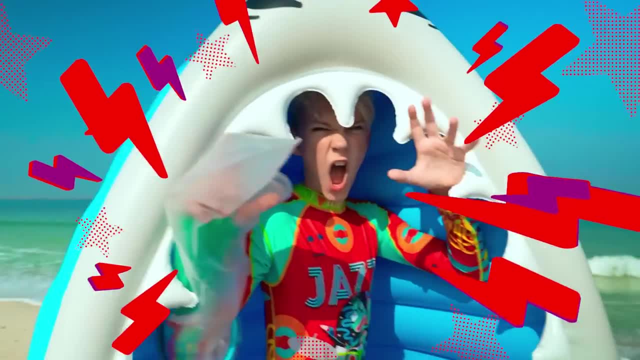 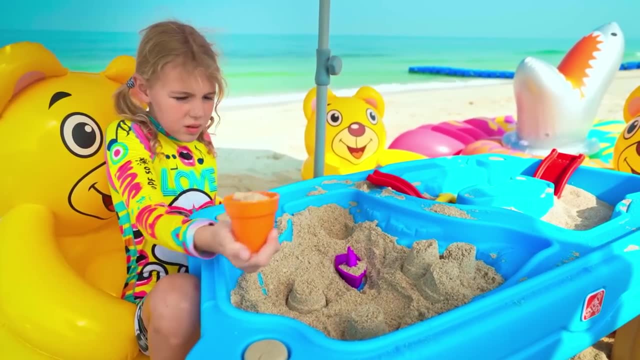 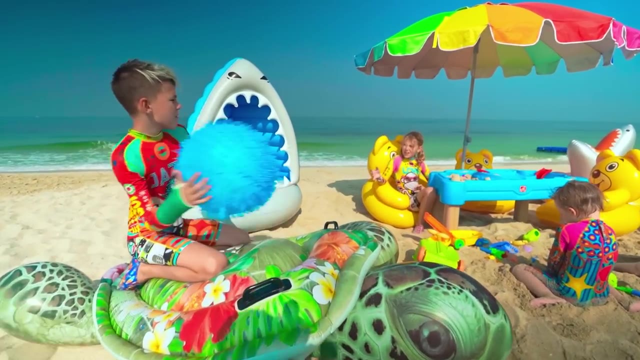 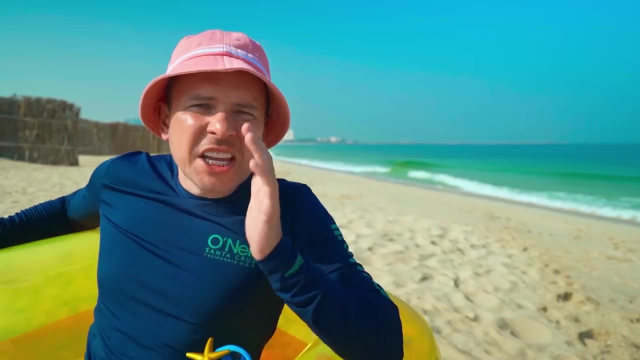 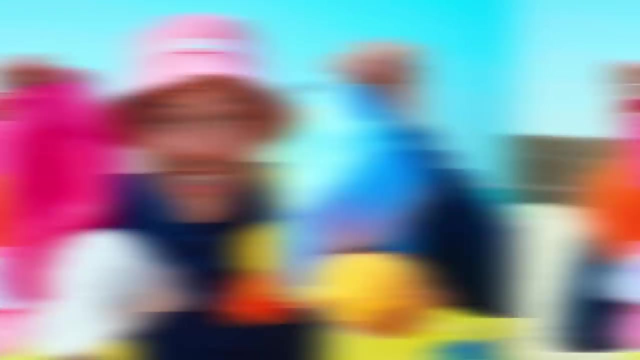 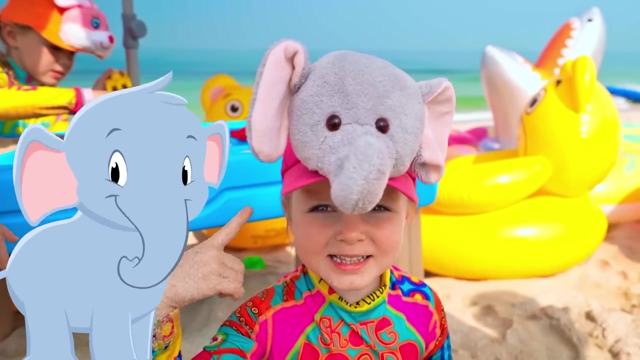 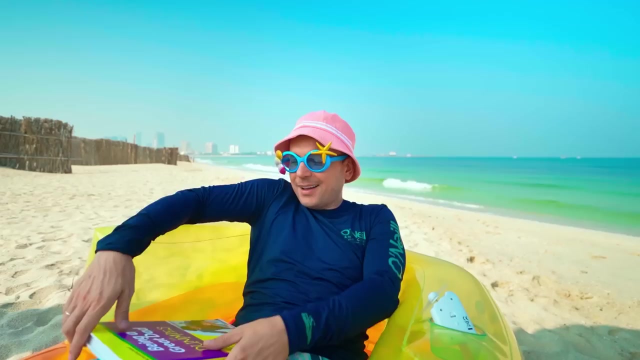 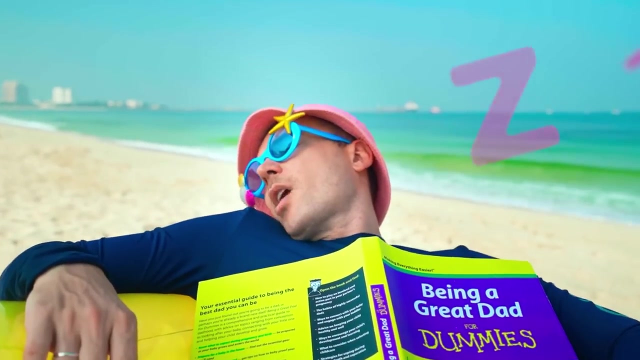 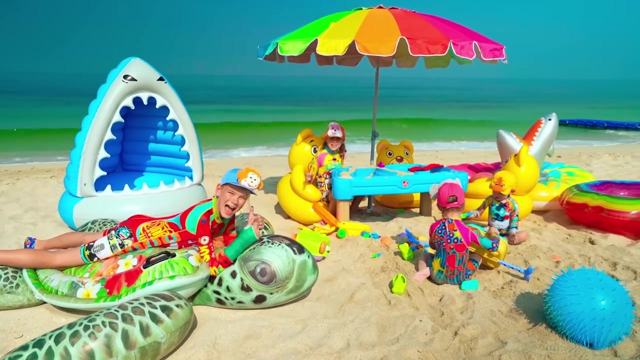 Kids put the hats on. We don't want. How about these funny hats? We like these hats: Monkey, Rabbit, Rock, Elephant. Aha, Nice, Let's prank our daddy. Yay, OK, OK, Woo-hoo. 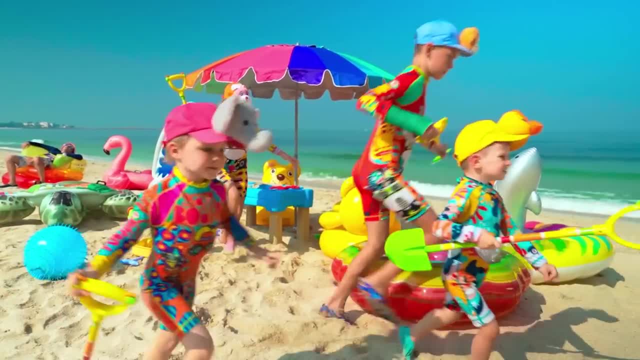 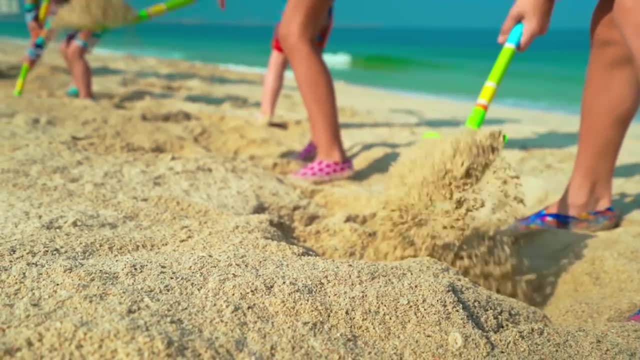 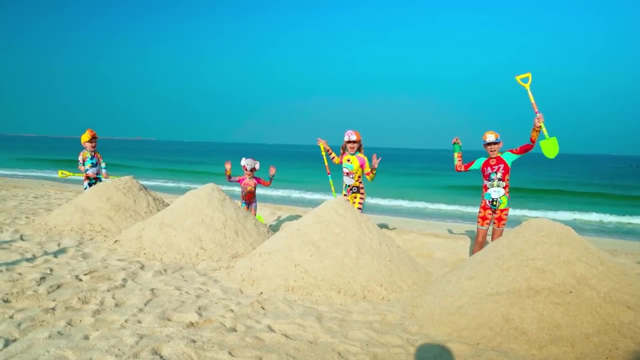 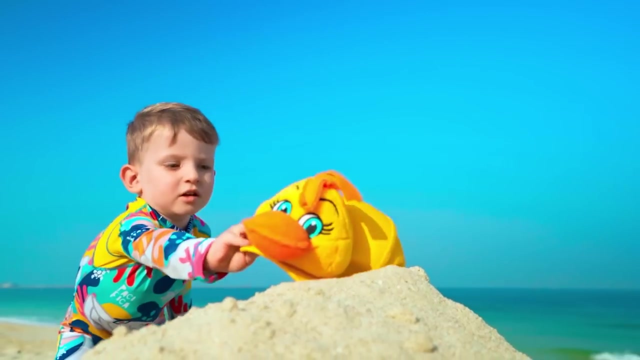 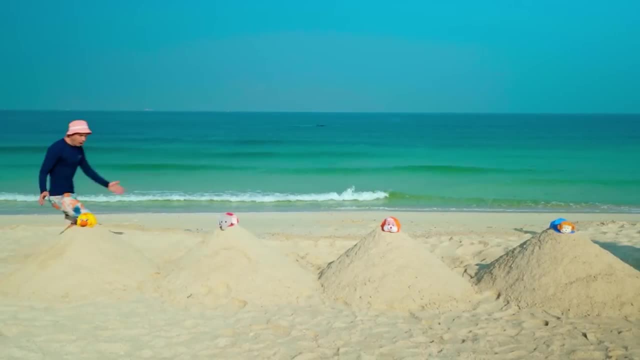 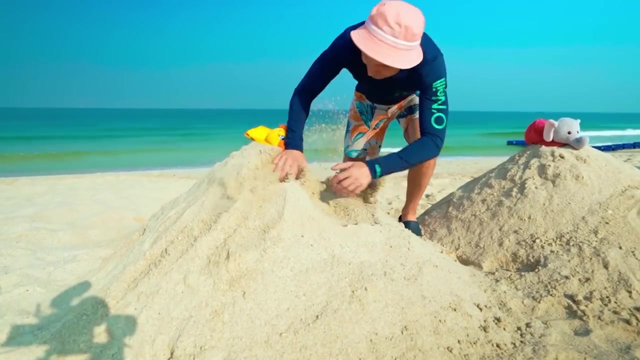 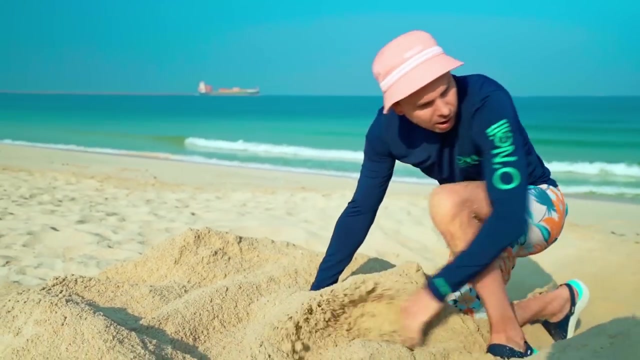 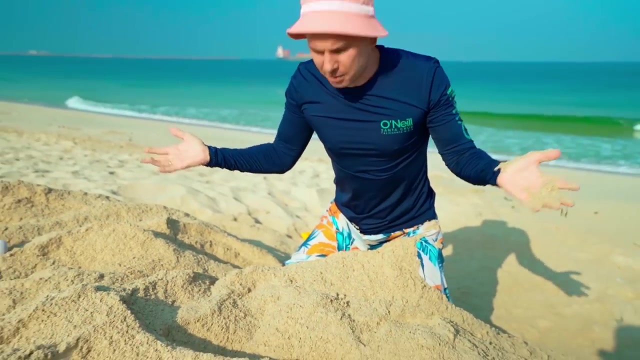 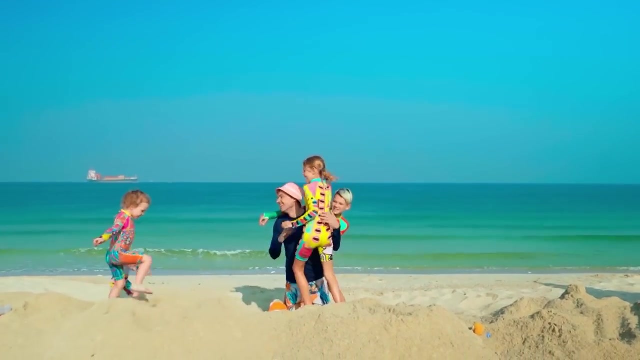 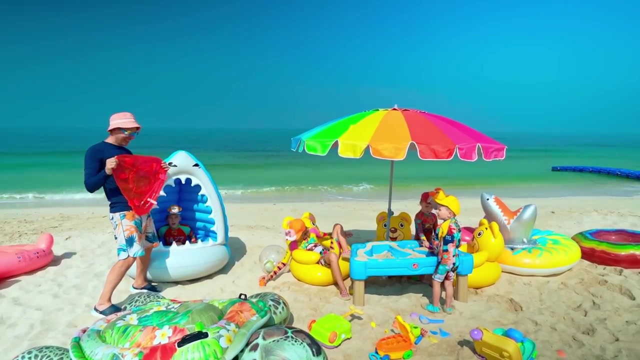 Daddy, Uh-oh, Uh-oh, Kids, where are you? Nobody's here. Uh-oh, Where are my kids? Where are they? Kids, check it out. What's this? It's a pumping house. You have to pump it. 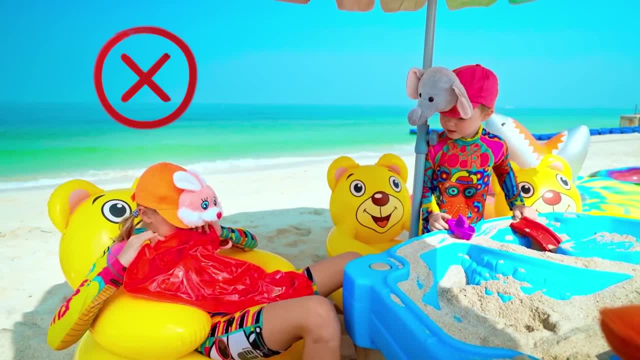 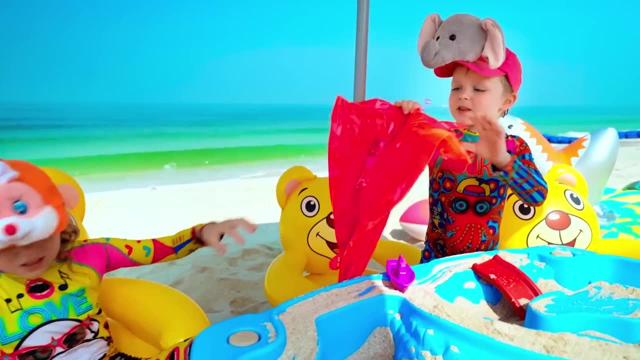 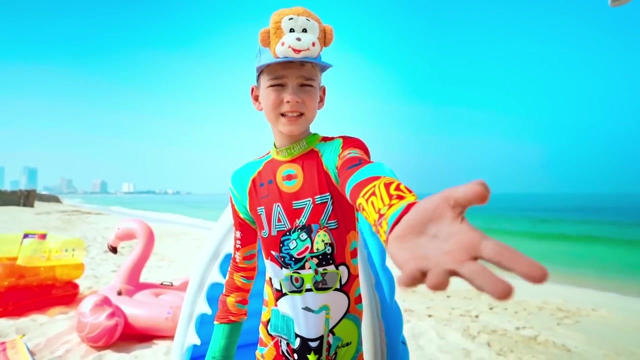 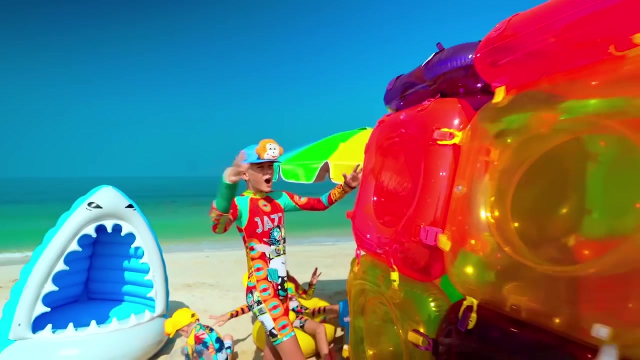 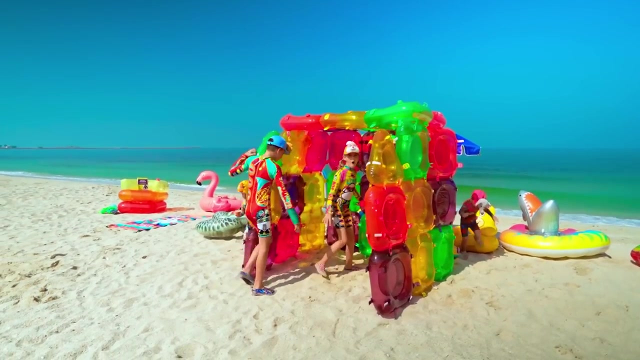 Wow, I can't. Let me try, Maria. Okay, Uh-oh, I can't. Girls, let me try, Wow. Guys, look what I have. Yippee, Wow, Uh-huh, Ho-ho-ho. 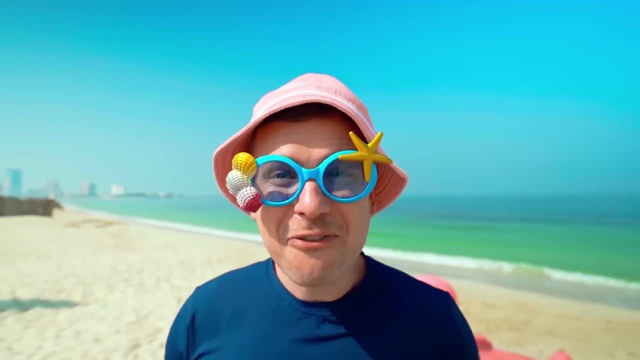 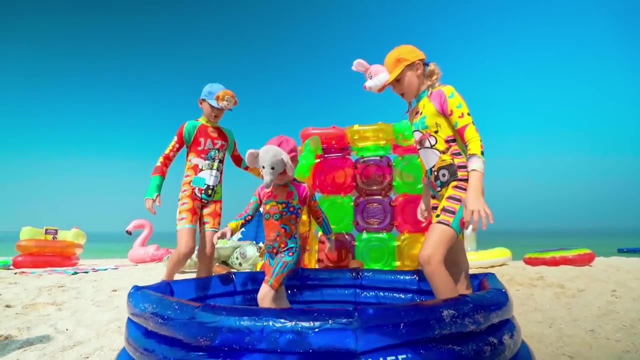 I have more fun stuff. Look, Woo-hoo-hoo, Stop, Stop. And who is hungry? Look what I've got. Yes, we are hungry. Uh-huh, Ho-ho-ho, Yeah, Uh-oh. 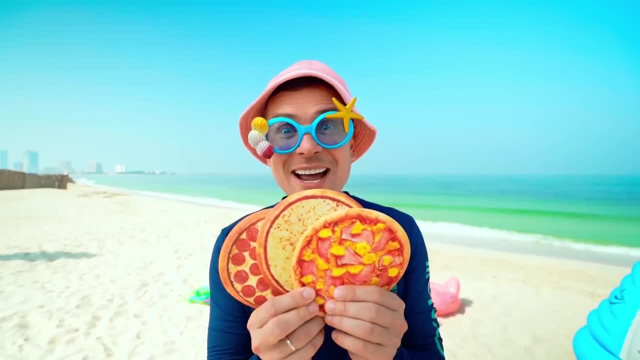 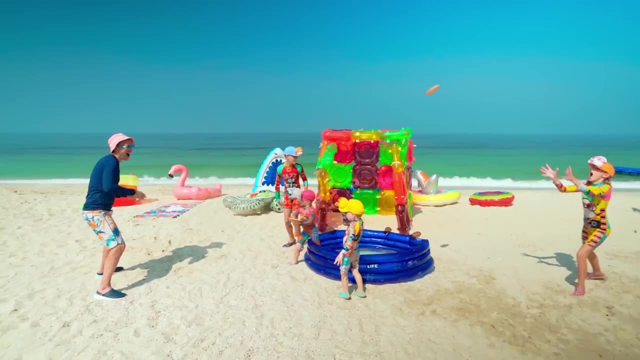 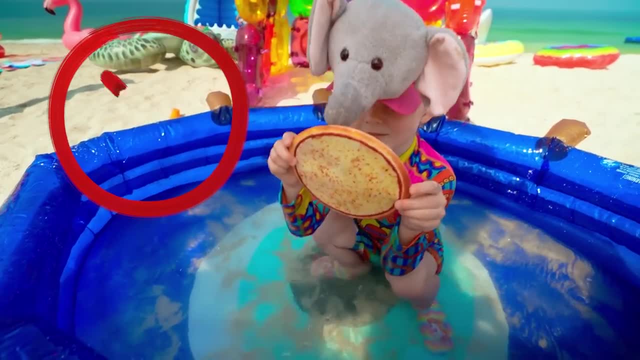 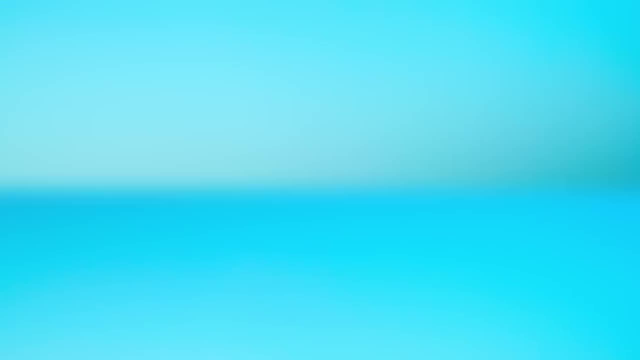 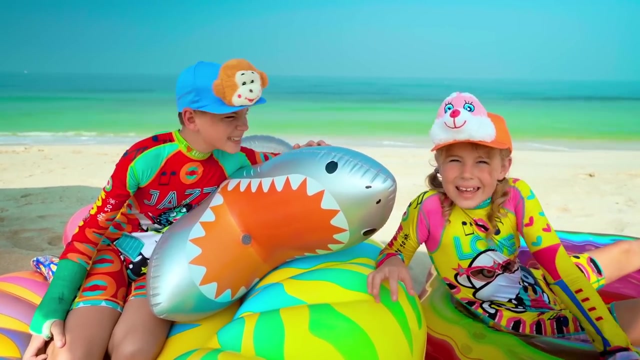 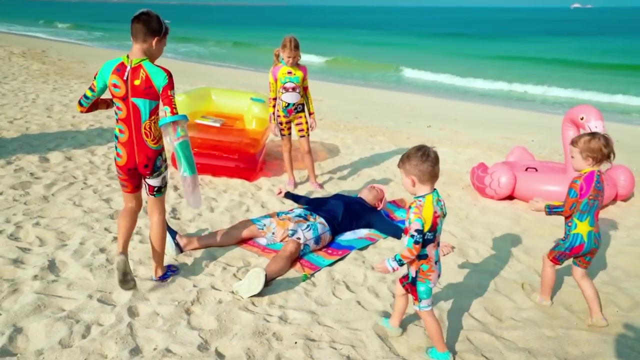 Uh-oh, It's not real pizza. Ha ha, It's fake pizza. Got you, Let's bury daddy in the sand. Yeah, Let's go. Ha-ha, Ha-ha, Yippee, Uh-huh. 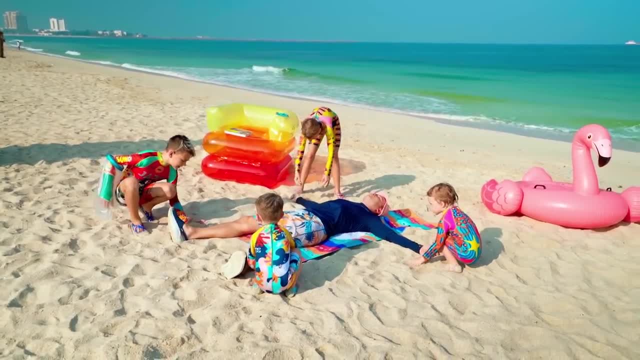 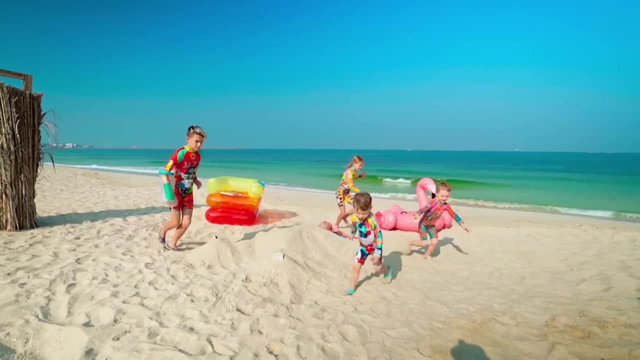 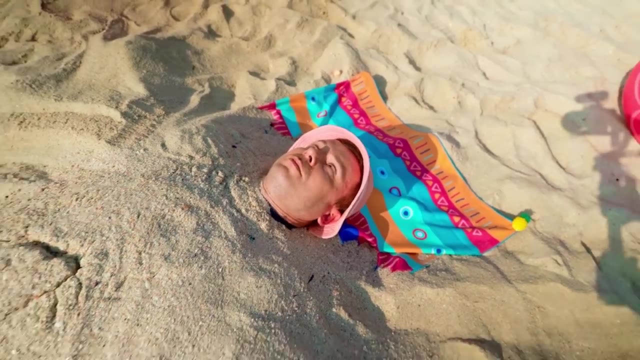 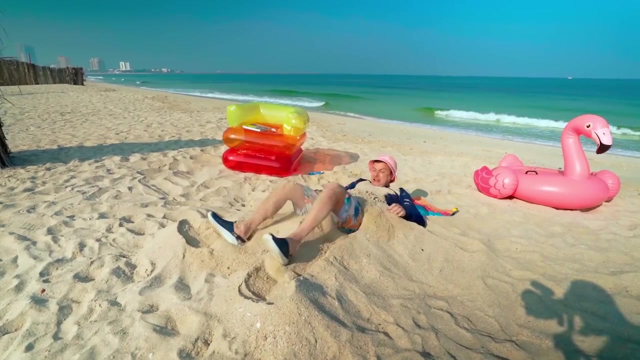 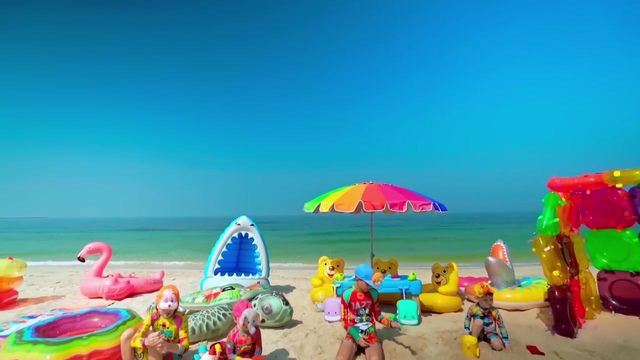 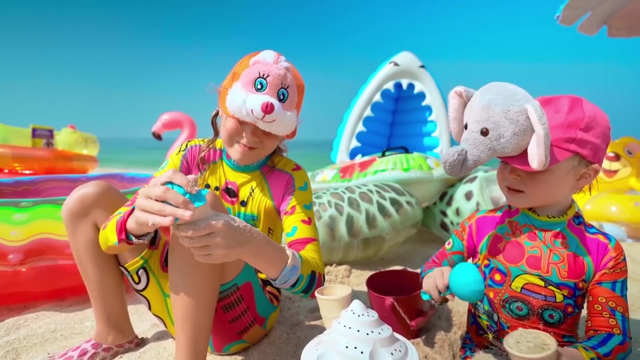 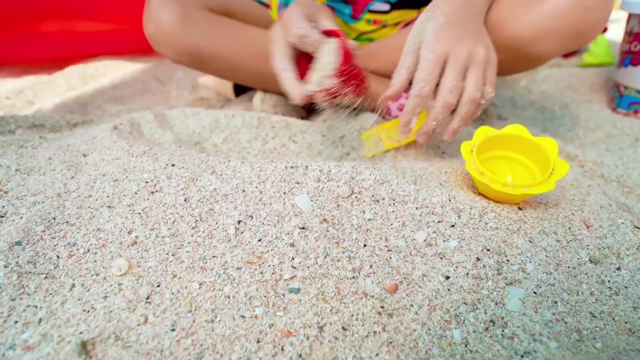 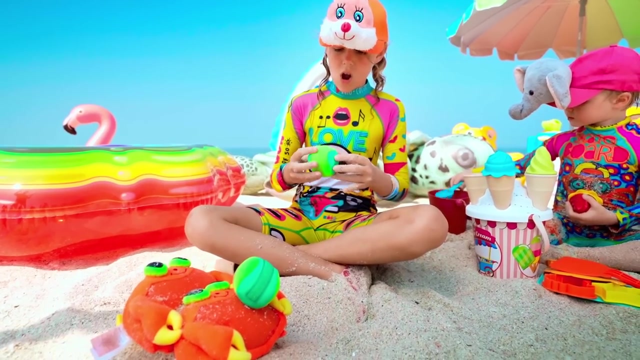 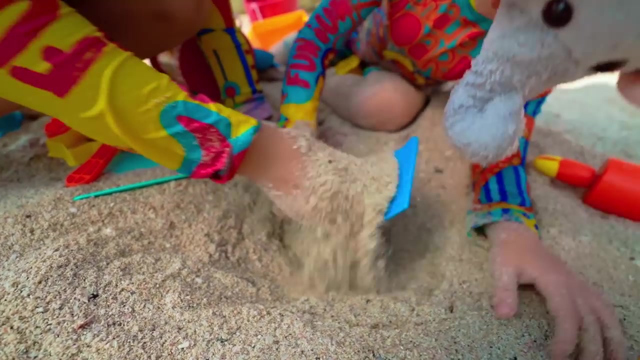 Uh-huh, No, no, no kids, Do you want sand ice cream? Yes, Ta-da, Your ice cream is ready. Thank you, Maria, You're welcome. Wow Idea, This is a set for a builder, Yeah. 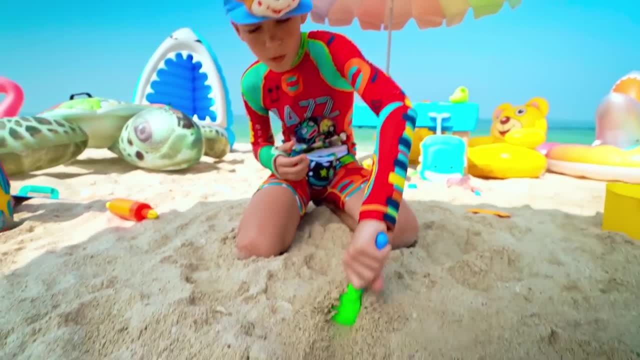 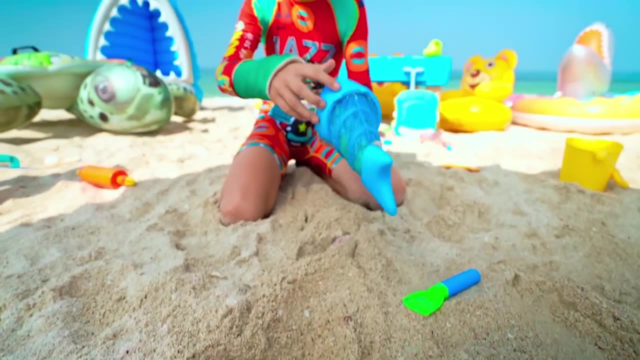 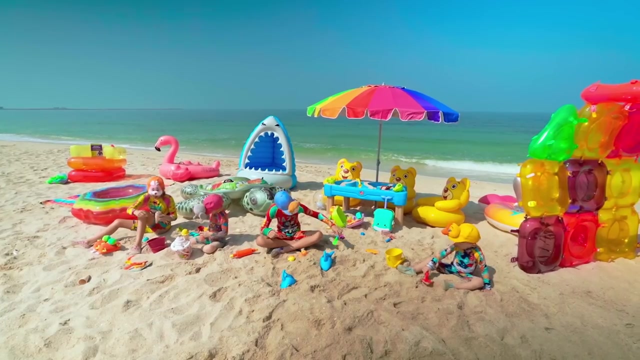 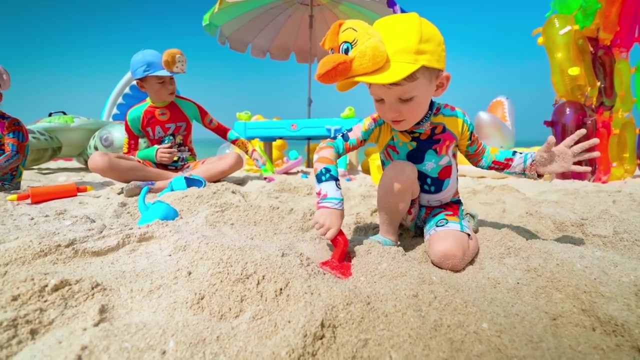 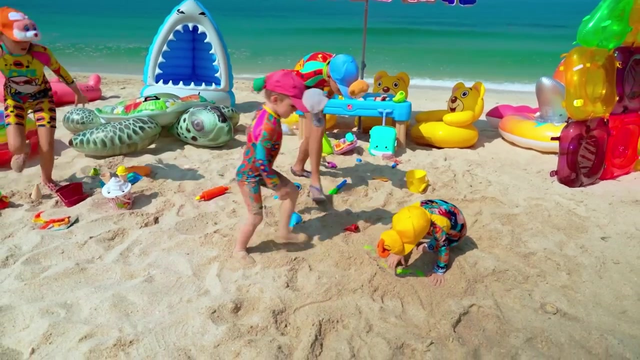 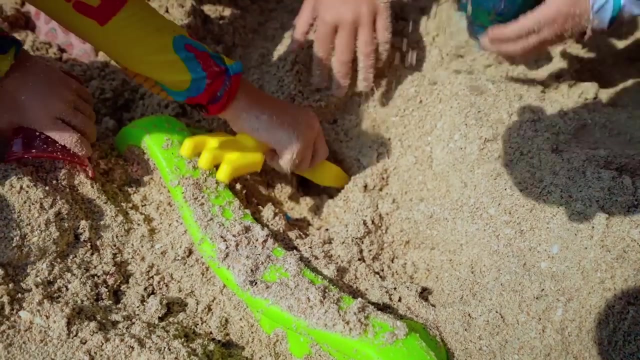 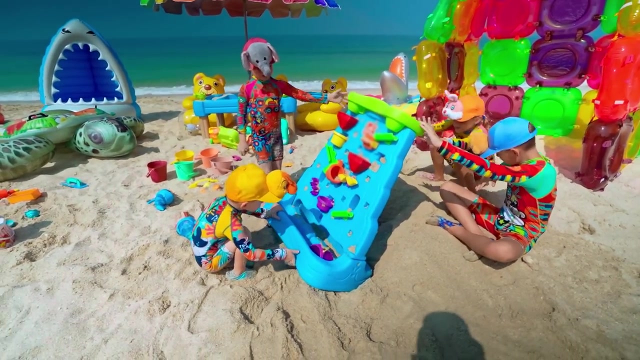 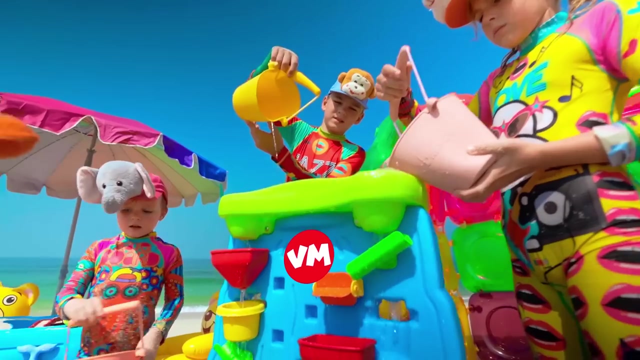 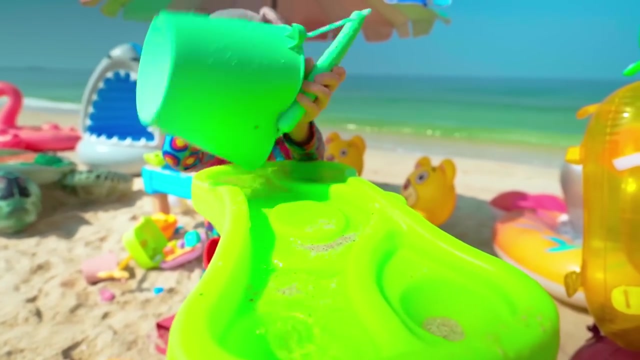 Maybe I will find something too. Wow, What's this? Woohoo, Wow, I want to do this. What's this? Yay, I found something. Guys, help me. It's something big. Wow, Wow, Help me, Help me. 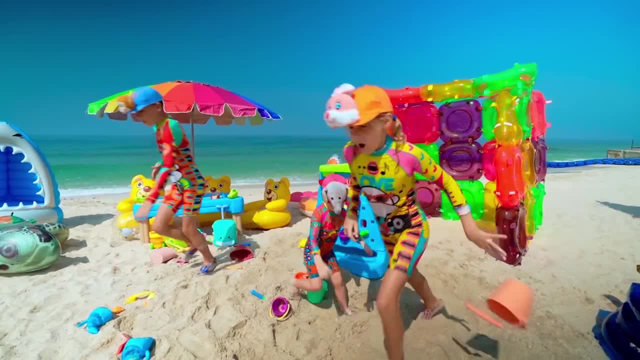 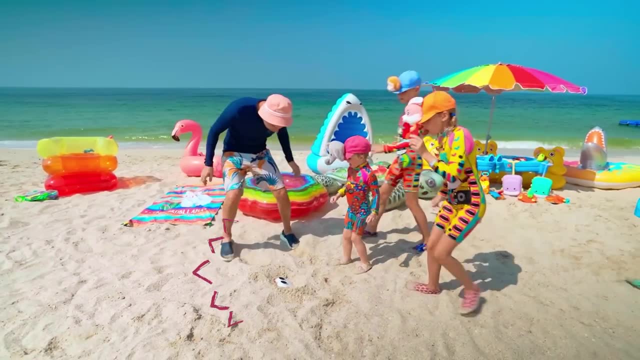 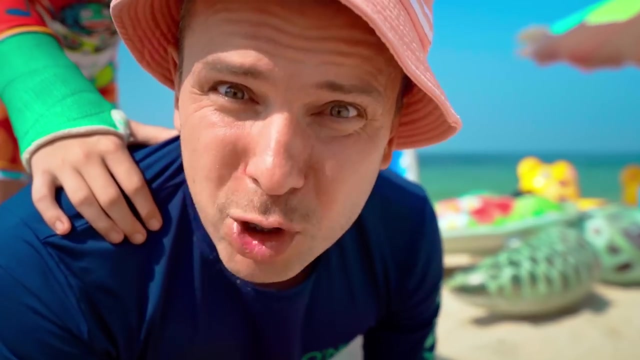 Help me. What's the sound? Help me? Who said that? Help me? Help me? It is: help, Let's go. Help me. Help me, Let's pull it out. Help me. Hmph, Huh, Oh. 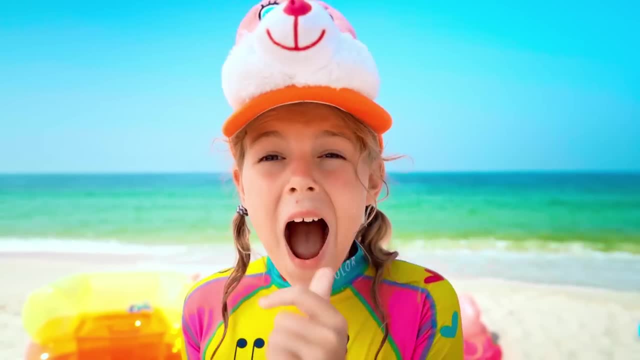 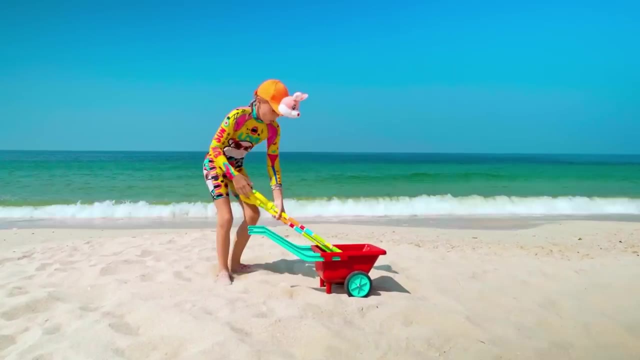 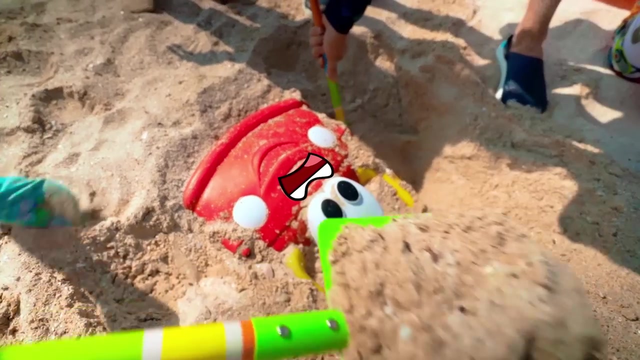 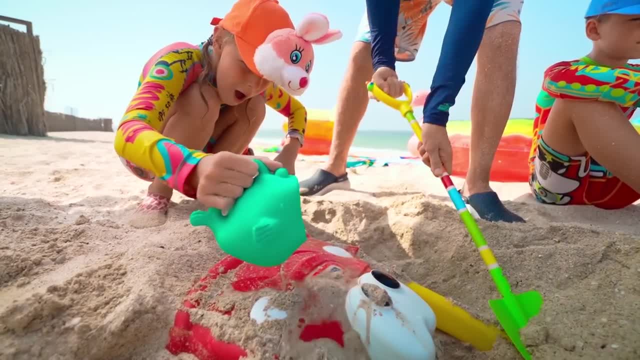 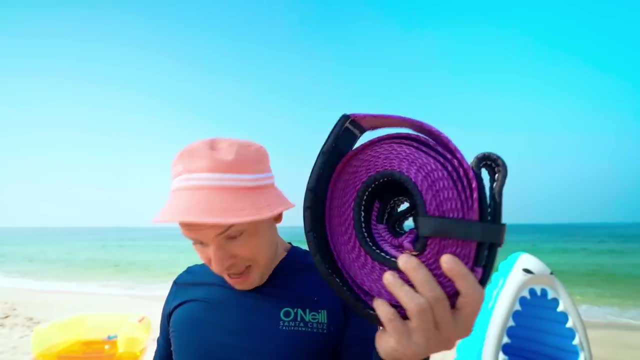 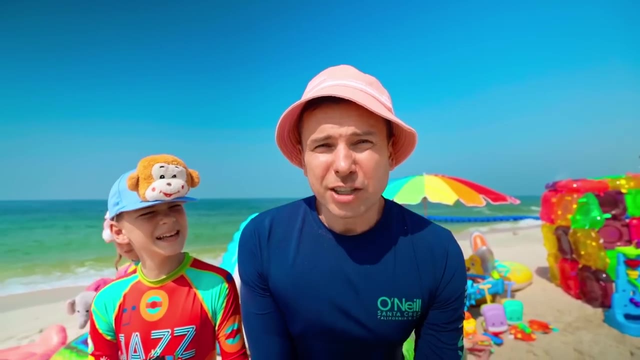 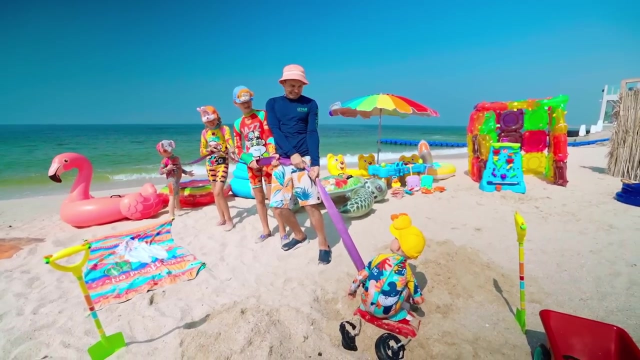 Oh, Oh, Oh, Oh, Are you thirsty? It takes too long… I need something special… And I've got some. Are you ready, guys? Three, Two, One, Push Hrmph Alex, What are you doing there?